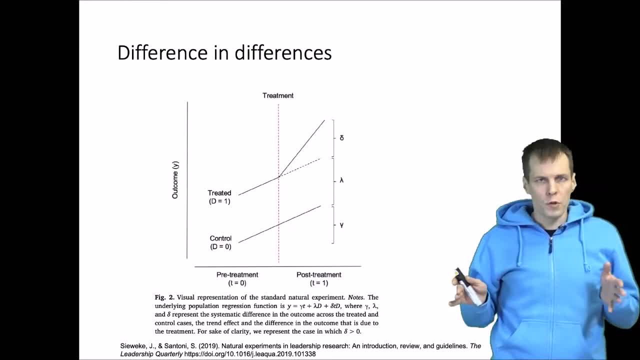 works is that we measure two groups. We measure both groups before the treatment and after the treatment and no randomization is required. And the name difference in differences comes from the main idea of this technique. So the idea of the technique is that we first calculate the difference before the treatment. here 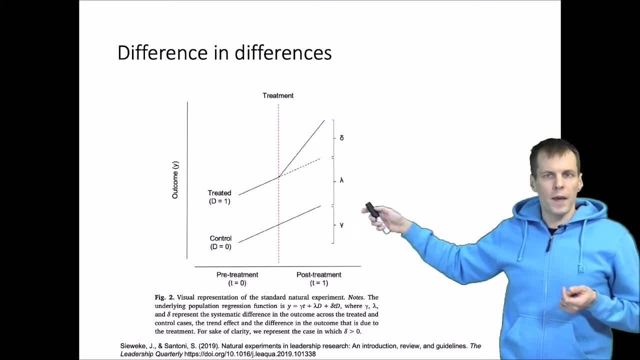 calculate the difference after the treatment and then difference in those differences. here the Delta is the causal effect. So if the difference between the treatment and control grows over time after the treatment, then we conclude that the treatment had a positive effect. If the difference between the treatment and outcome decreases or becomes more negative over time after the 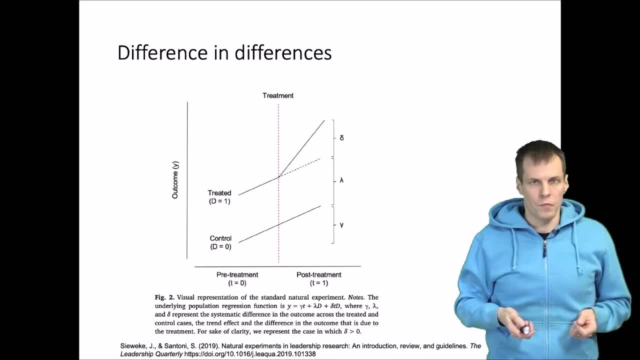 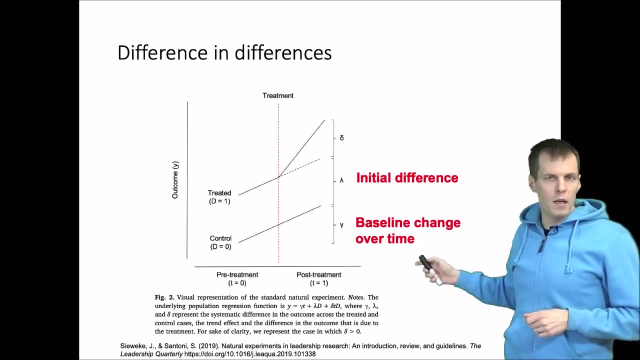 treatment. then we conclude that the causal effect is negative. So here we have our lambda, the initial difference. so that's the first difference. Then we have baseline change over time. We are typically not interested in this baseline change over time, but that would is the. 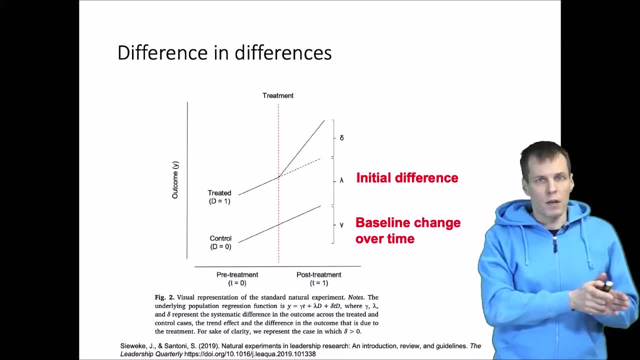 change that prevents us from just comparing the treatment group against itself before and after the treatment. and then we have the treatment effect Delta here. So how do we? how do we then do this in practice? We could calculate the two differences and then subtract them, but the 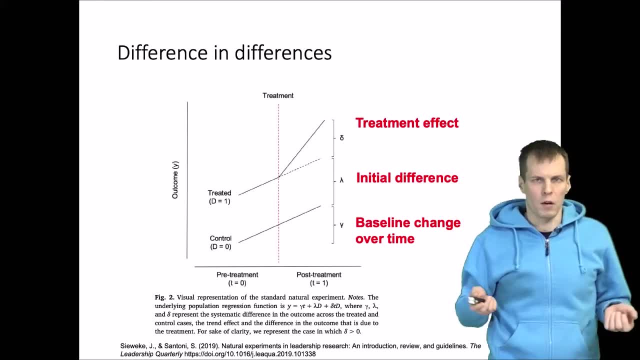 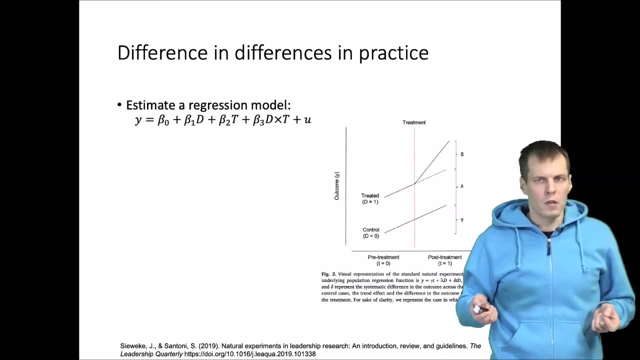 problem is that if we do that in Excel, for example, then how would we calculate the standard error? In practice, this analysis is typically carried out using a simple regression model. So we have a regression model here, We have the D, the treatment, T, the time, and then we have beta one for the. 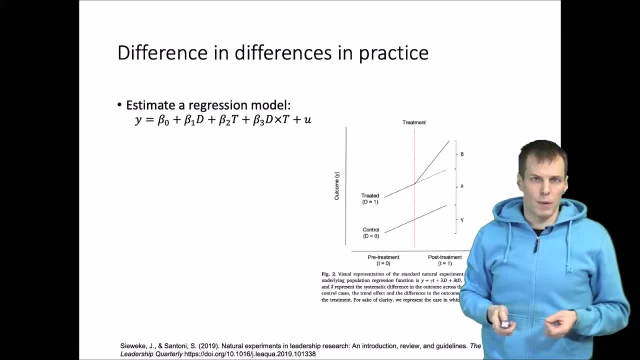 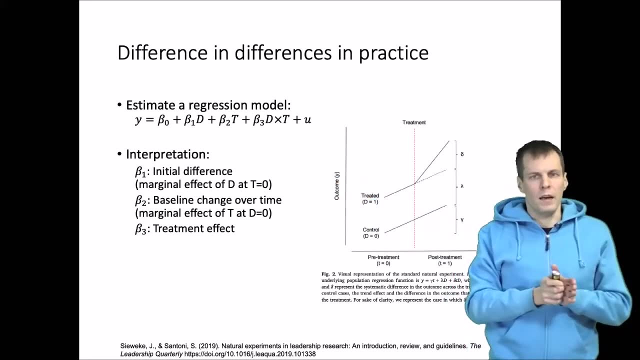 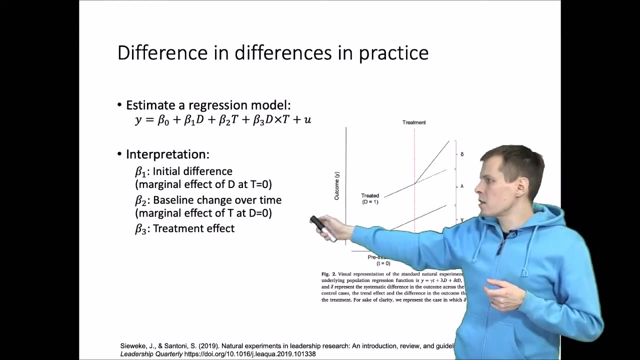 the treatment, beta two for time and then interaction between treatment and time. And how do we interpret this? Well, beta one is the initial difference. marginal effect of D at T is zero. So that's the difference between before the treatment and then we have. beta two is the baseline change. 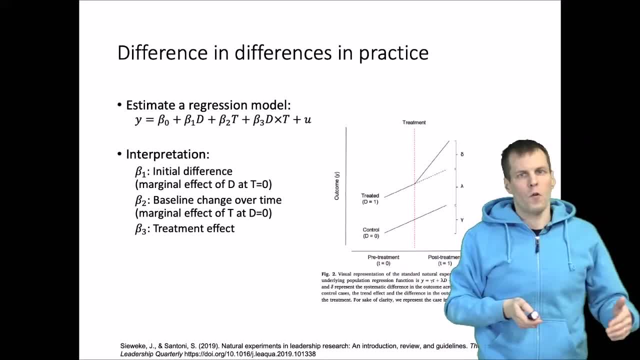 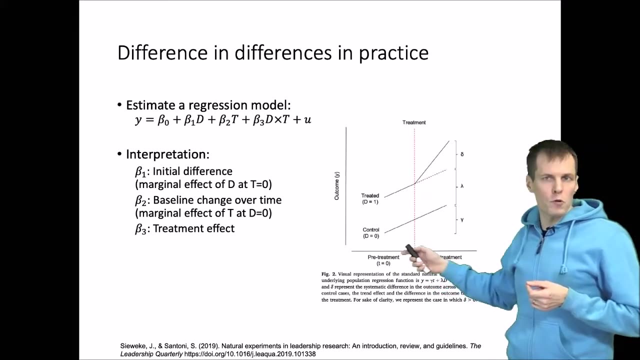 over time. So it's marginal effect of time for the control group. and then beta three is the treatment effect. It tells us how much the difference between the treatment and control increased over time when we went from from post, from pre to post treatment. So very simple So. 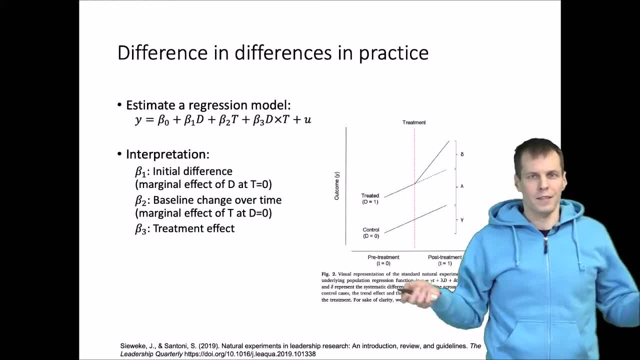 you just need two variables and their interaction and then you have a causal effect. Of course, if that will also always give us causal effect, the life of a researcher would be very simple, but it does not. It requires some very strong assumptions and we need to understand those assumptions and 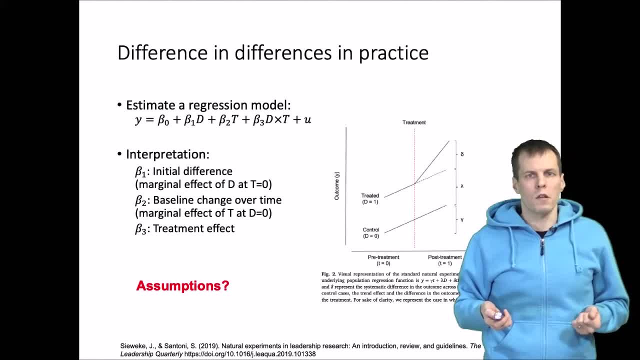 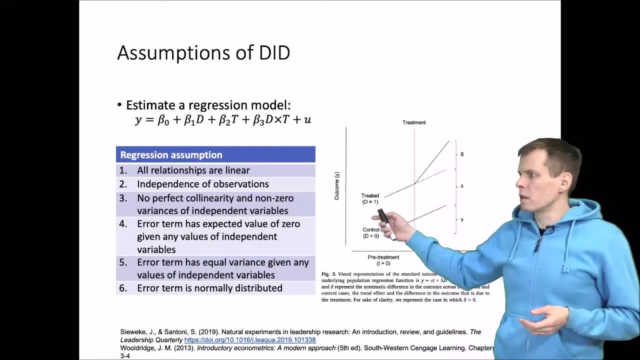 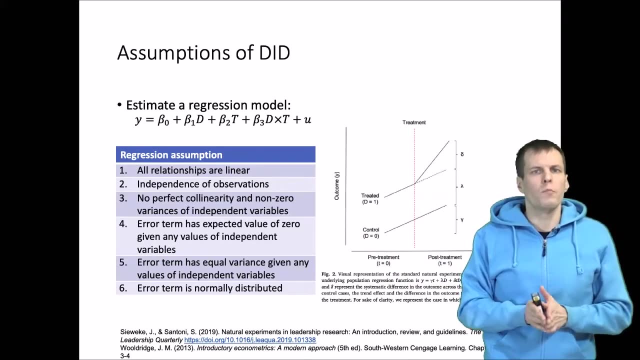 then also justify those assumptions in our article. to actually this technique produce any valid causal estimates? Because this is simply a regression model, it's useful to start with the regression assumptions. This is from Woolridge. We have six different assumptions and not all of those are equally important. Let's take a look at which assumptions. 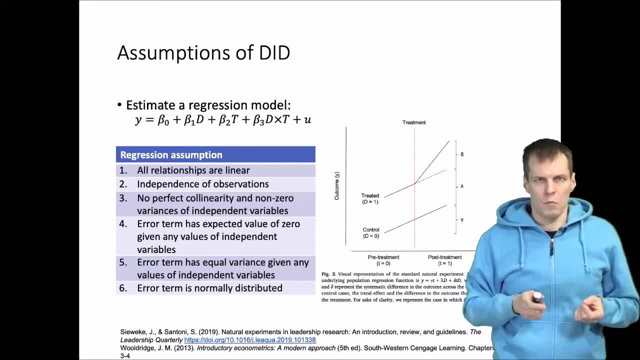 are possibly violated and one of the assumptions is always violated and that's difference in differences analysis. When you read about difference in differences of the explanations or introductions, you can see that the difference in differences analysis is very important. So it's clear and true and true how the difference is detected. 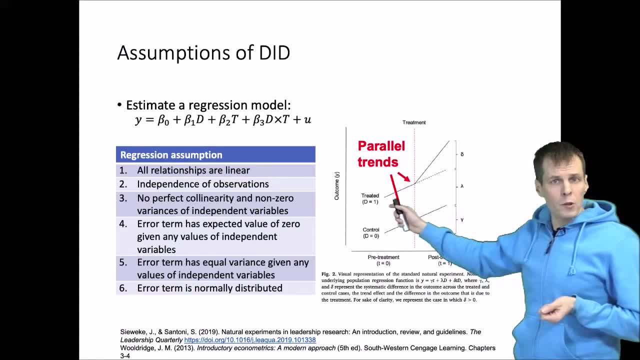 Because you should continue gonna go for that result, and you have to, tôi have to�. When you read about differences analysis, then of course you have to add this data to make an more precise picture. So here the evidence that was reported in the paper used. 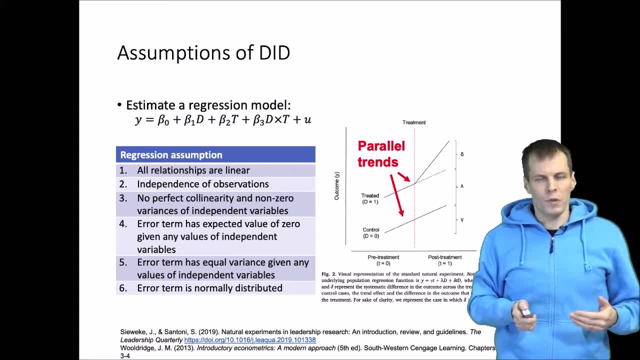 also in fact is from material analysis. So be aware of some of these Nazim's values here. the same way over time as the control group did, had the treatment group not received the treatment. So the development of the control group is used as counterfactual for the development of the. 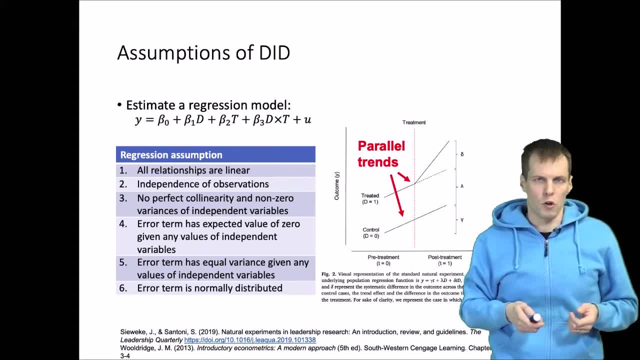 treatment group had it not received the treatment which we don't really observe. And this is critically important assumption, because if the parallel trends assumption does not hold, then our estimates will be inconsistent and causal inference will be invalid. So, for example, what would this parallel trends mean? Let's assume that we have a medical trial, we have sick people and we 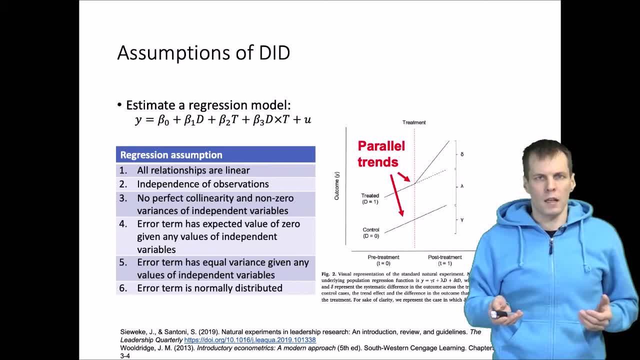 have healthy people, and then all the healthy people decide that they will go for the control, all the sick people decide that they will go for the treatment. and then we compare the health over time. If people didn't not get sick spontaneously, or even if people did not get cured or get well spontaneously, then there 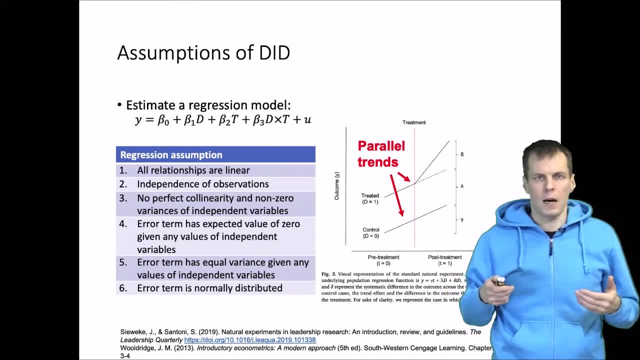 will be no trend over time. so and any difference after the treatment will be a result of the medication. So in other words, if the medication is the only reason why people could get well, then we have a clean causal estimate. But that's not, of course, the case if we have people that are first. 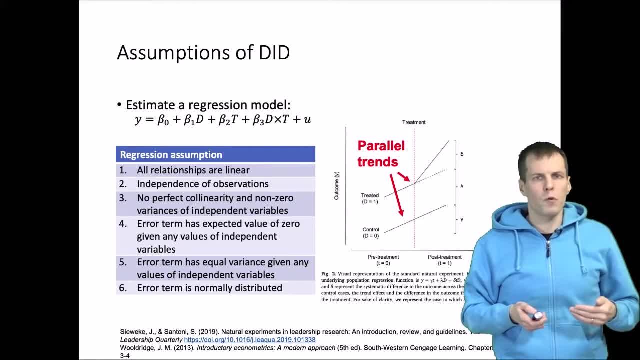 sick to start with, some of those people will get better over time, even if they did not have their own medication. So the average health of people who are sick to start with is probably going to increase over time. Also, if you have people who are healthy to start with, some of those people will get sick during that. there are the 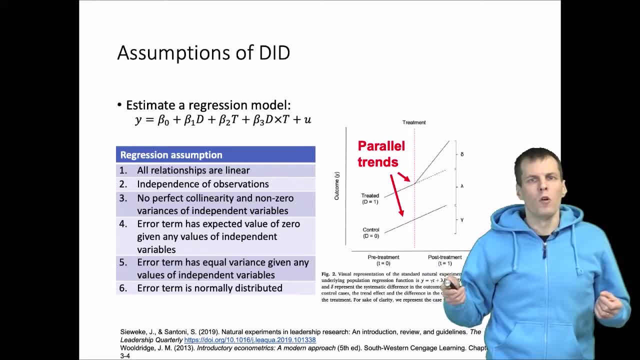 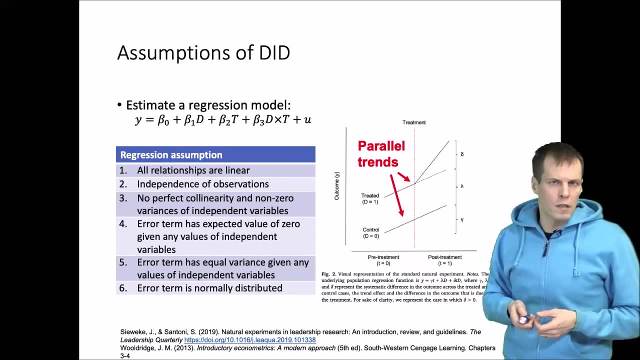 study period. so on average, those people, their health, will decrease over time, And that's an example of scenario where the parallel trends does not hold. So which of these regression assumptions is violated when the parallel trends assumption fails? Let's take a look at the regression. 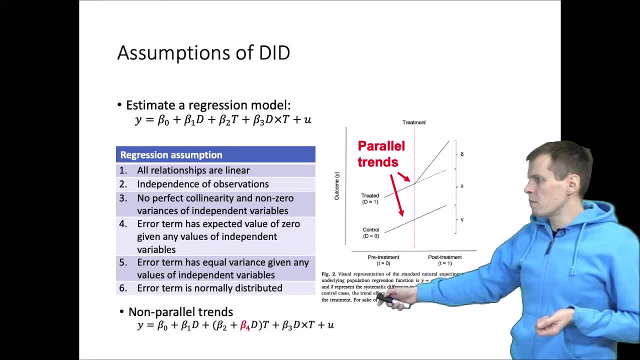 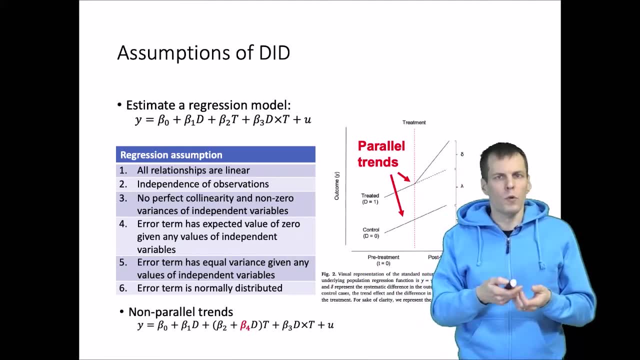 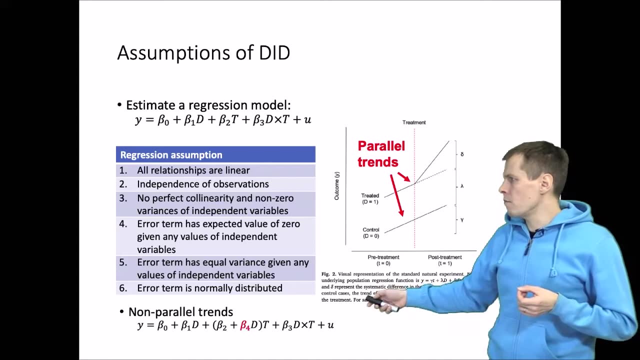 request. So if we have a non-parallel trend, it means that the effect of time t would be different for the treatment, even if the treatment group would not get the actual medication or whatever the treatment is. And if we reorganize this equation a bit, we can see that because we don't observe what would be the effect for. 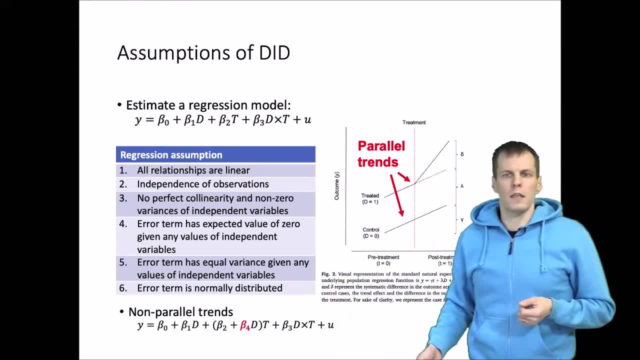 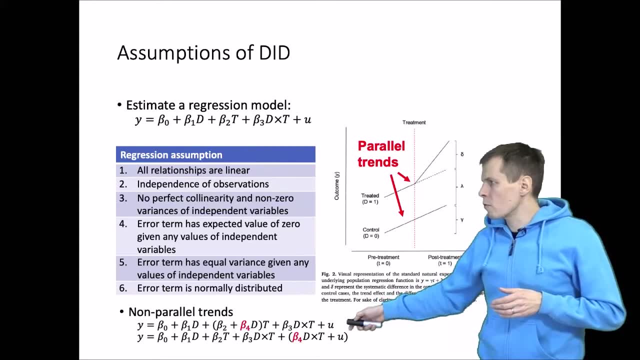 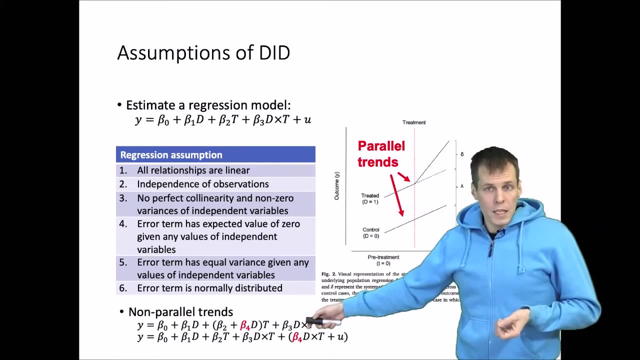 the treatment group had it not received the treatment. this is unobserved and it goes to the error term And we can see from this simple rearrangement that this error term, which includes the trend of the treatment group, had it not received the treatment, if this beta four is 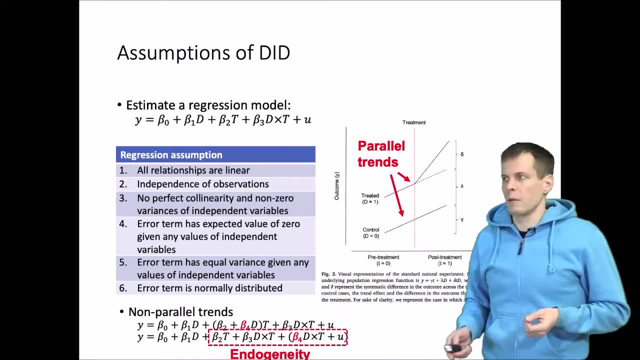 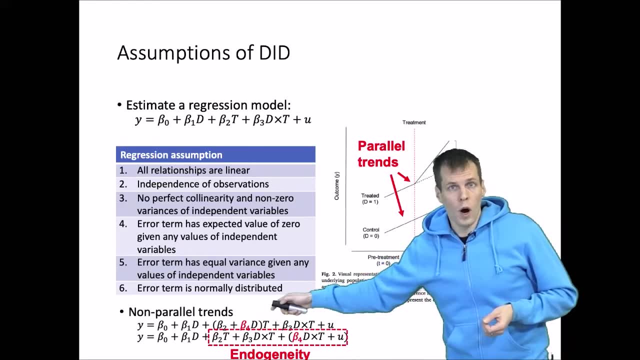 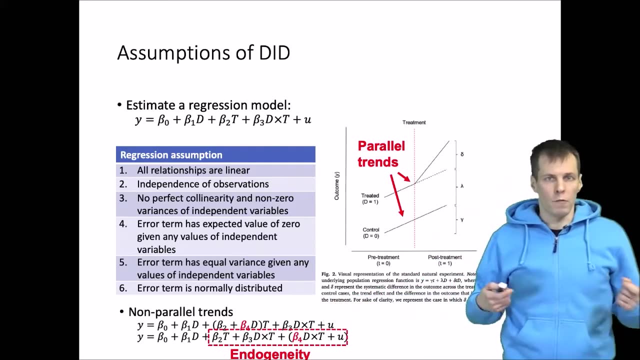 non-zero, which means that the trends differ. then we have an endogeneity problem, because this term here correlates over these two terms here that contain the t. Why it correlates is because beta four is non-negative if the trends are not parallel and d is one for the treatment. 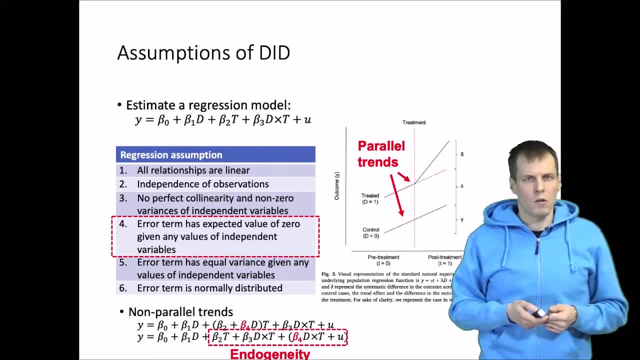 group. So we have an endogeneity problem unless the parallel trends holds. We have also another assumption that is violated and it is the non-independence or the independence of observations. and the observations are non-independent because we are measuring each person twice, before the treatment and after treatment, and there are probably some. 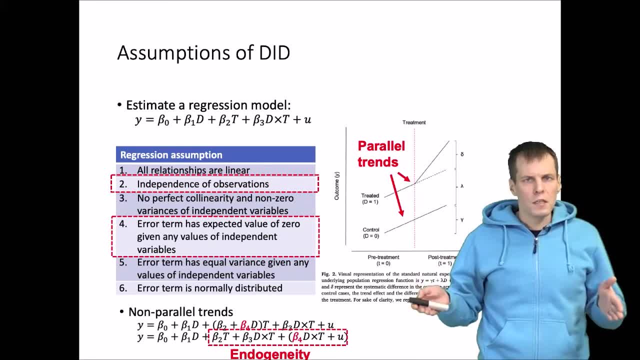 causes of the dependent variable that persist over time, so that if we measure one individual before the treatment and the same individual after the treatment, those two scores will be more similar to one another than if we measure one individual before the treatment and another individual after the treatment and then compare the differences. 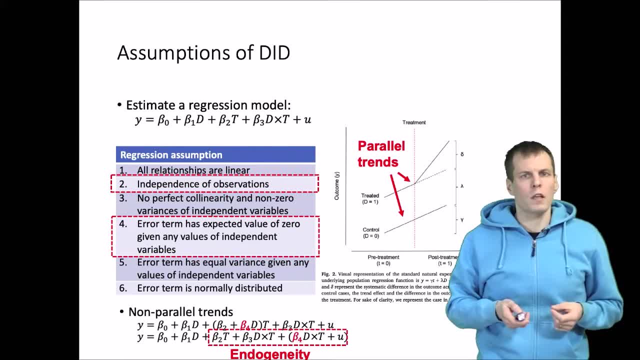 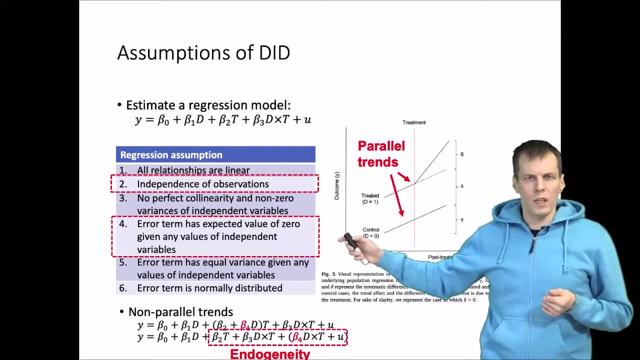 So we are in violation of that assumption. So these are the two critical assumptions in difference, in differences, and let's take a look at how they are typically dealt with. So so this has to be justified, the parallel trends and this violation has to be dealt with. 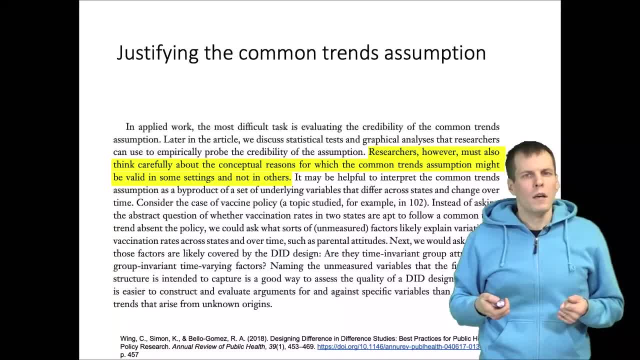 So the parallel trends assumption or common trends assumption can be justified in two different ways, and generally you should do both in your study. So first you should provide a conceptual argument based on theory: Why, Why do you think that the trends should be parallel? 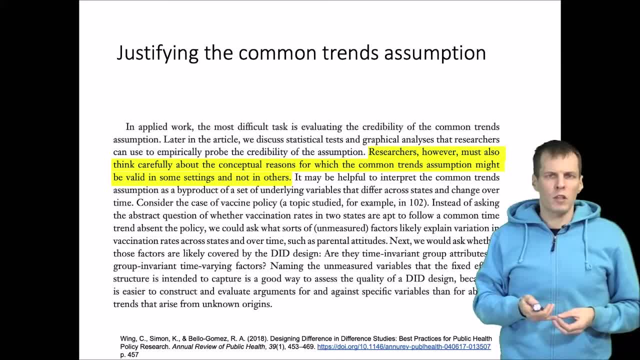 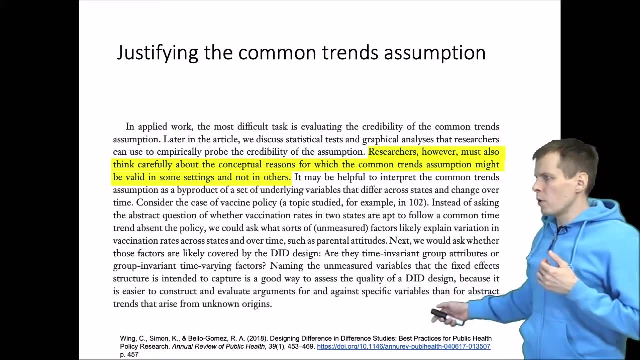 So if we think about, let's say, a person's health, how it evolves over time, we should start thinking about what causes differences in in the trends and then whether those causes are present and also different between our treatment group and control group. This article by Wing gives a pretty 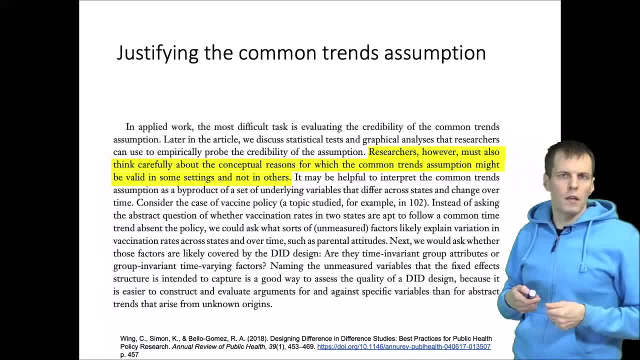 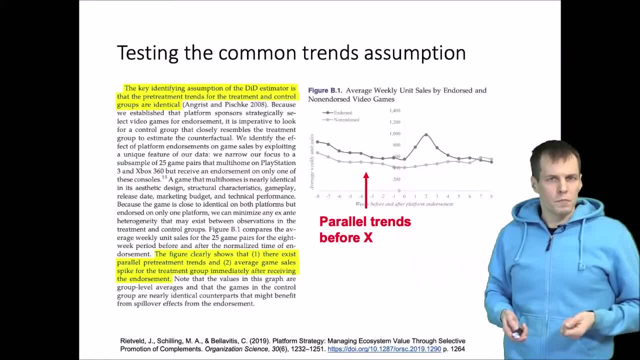 good explanation of how you could start arguing. there are the common trends or parallel trends assumptions conceptually, Then there are empirical ways of doing it, So you can test the common trends assumption, or let's say test, because it is ultimately untestable, but you can provide some evidence that it may hold and the idea of testing the common 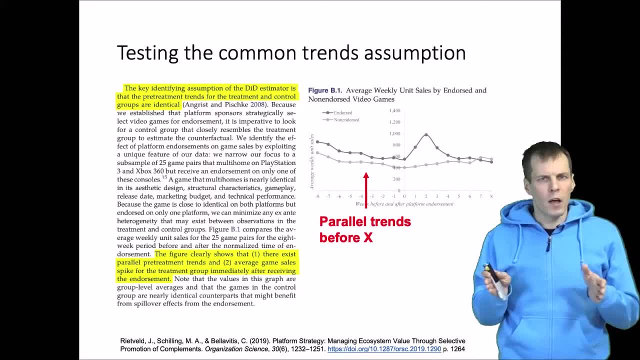 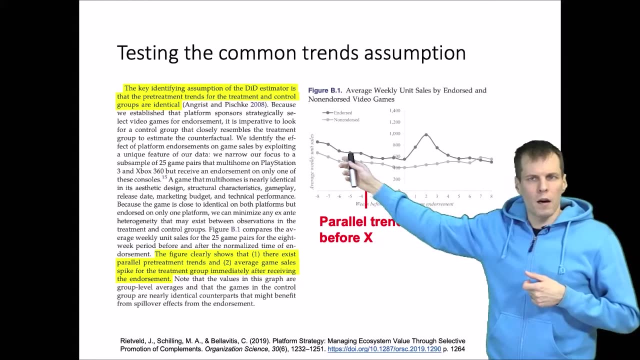 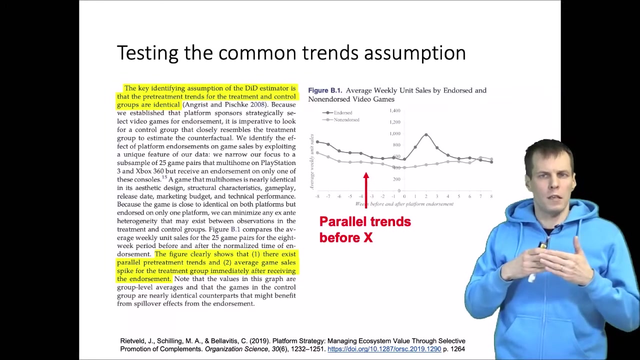 trends. assumption is that we compare how the trends develop before the treatment. So this is an example from from Wright Welch paper and they have two groups and they compare that both groups had the same trend. The treatment group was higher. but we don't care about the level differences, we care about the differences in 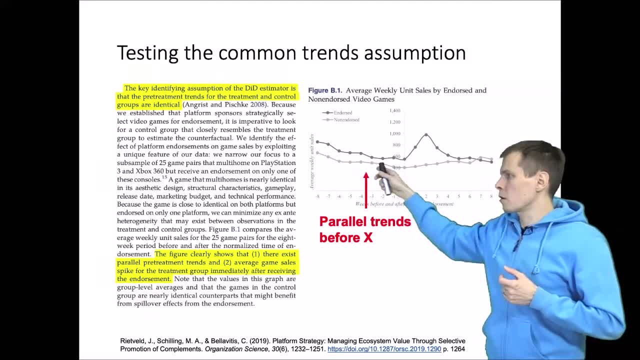 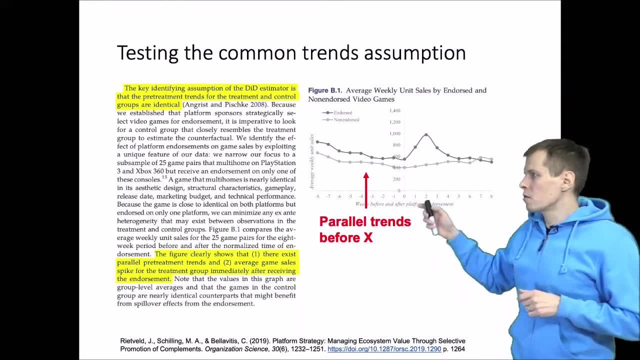 direction and these two trends. they follow each other quite closely. So, based on this figure, the authors argue that the trends appear to be parallel. So if the control treatment group were not in the treatment, they would probably have been developing somewhere over here.